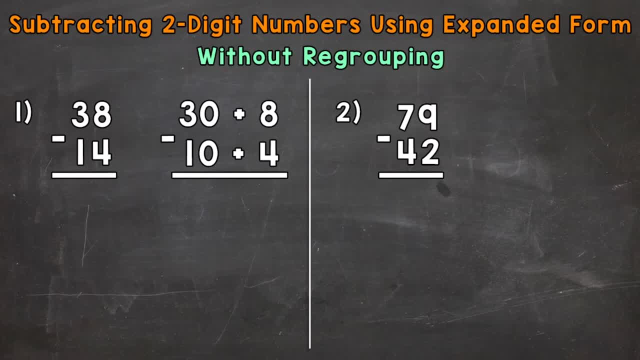 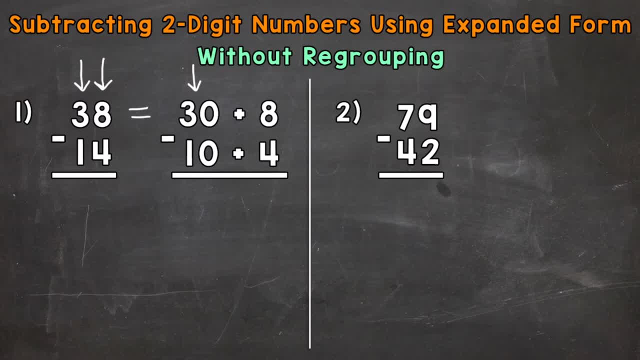 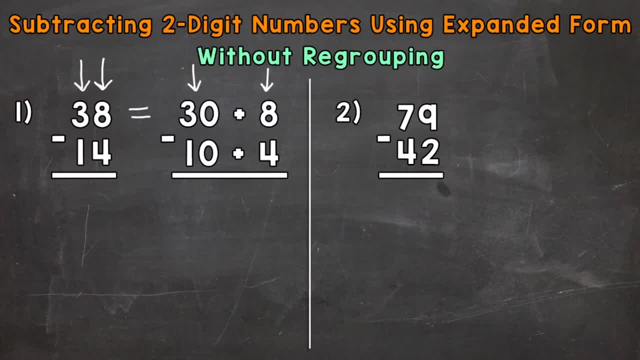 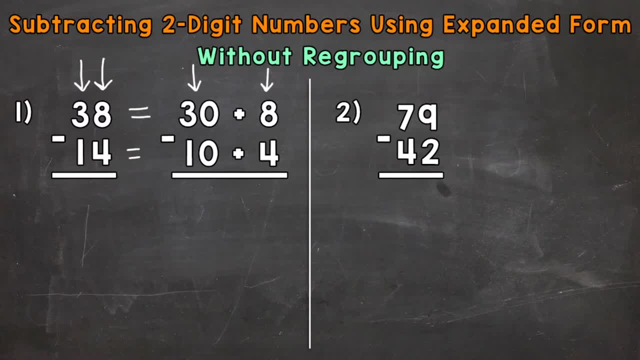 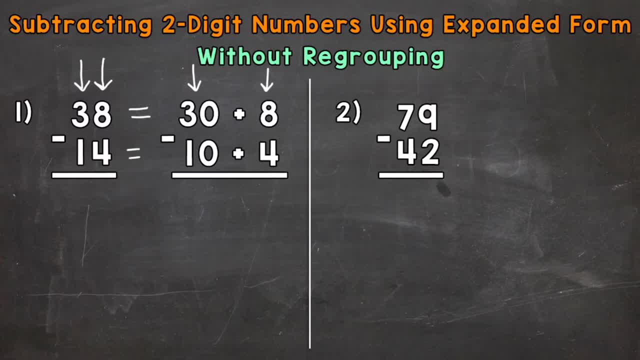 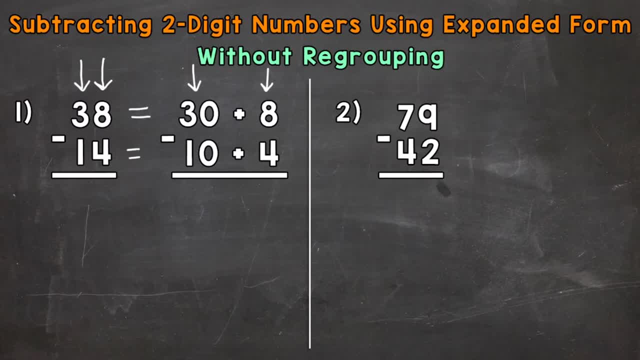 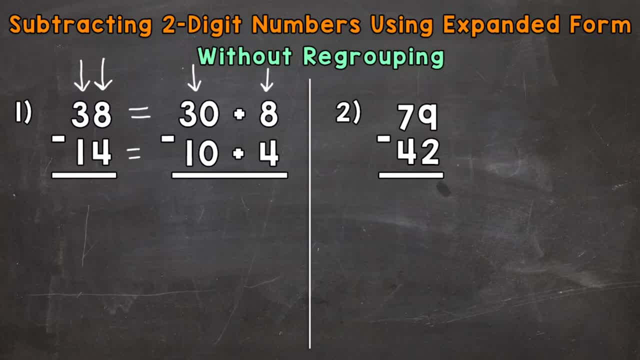 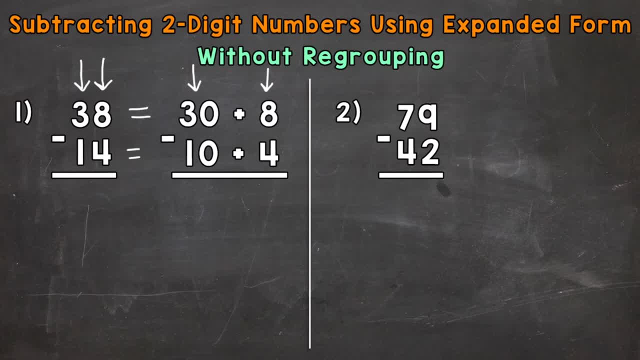 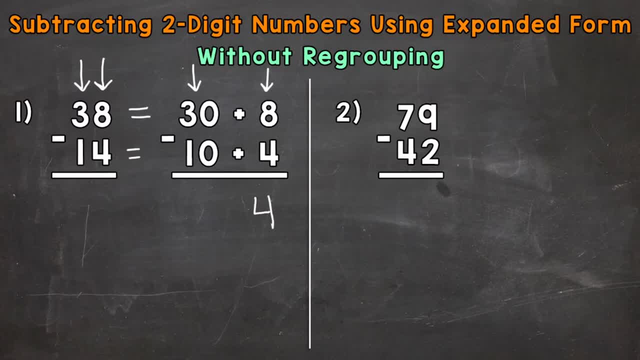 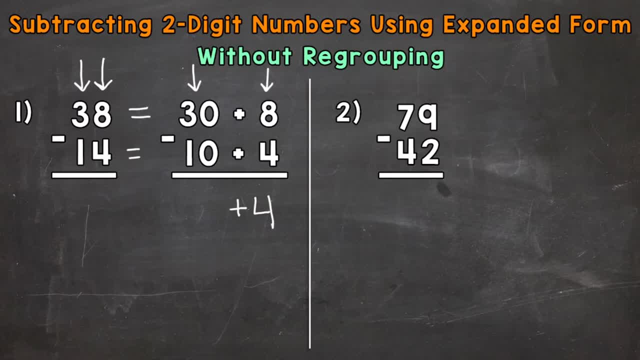 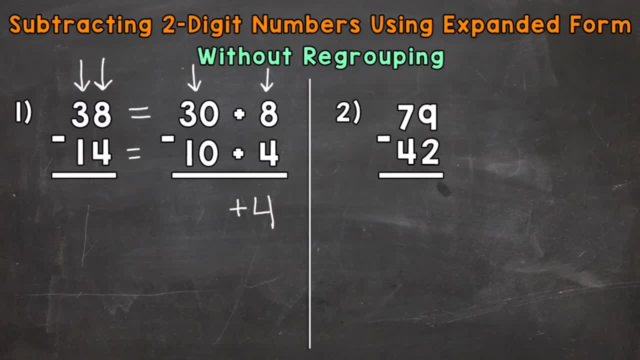 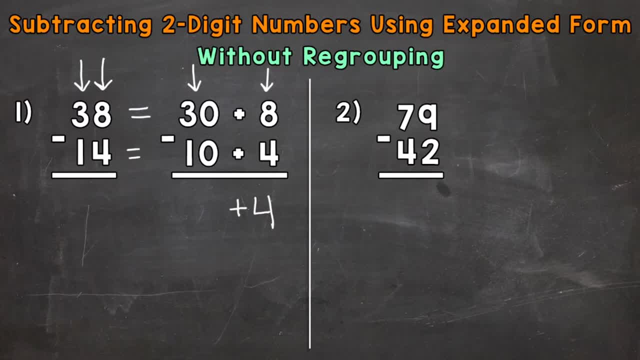 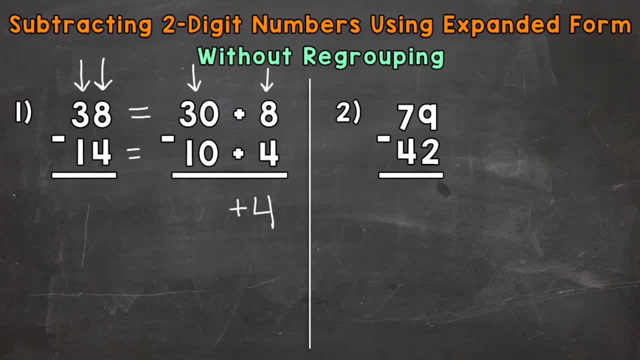 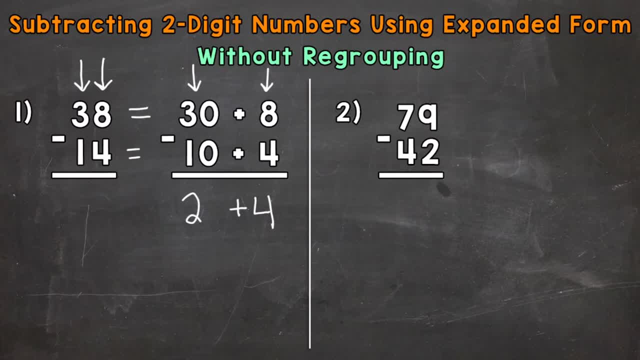 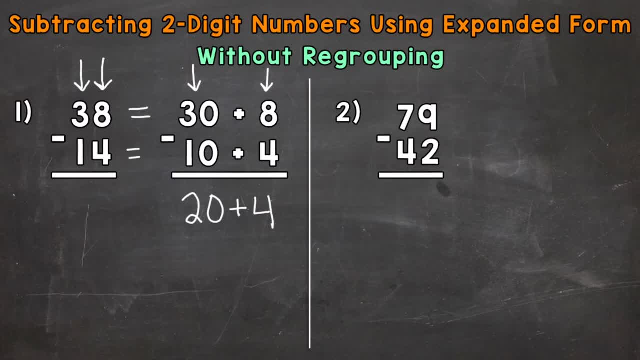 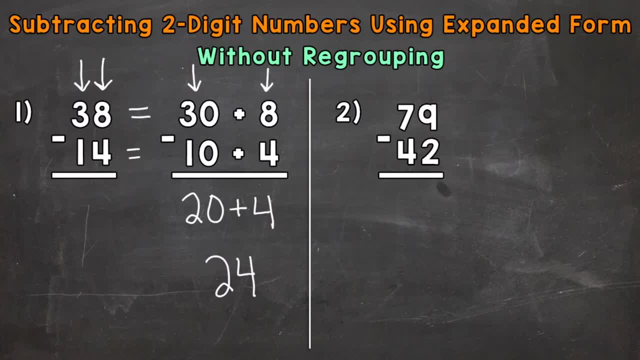 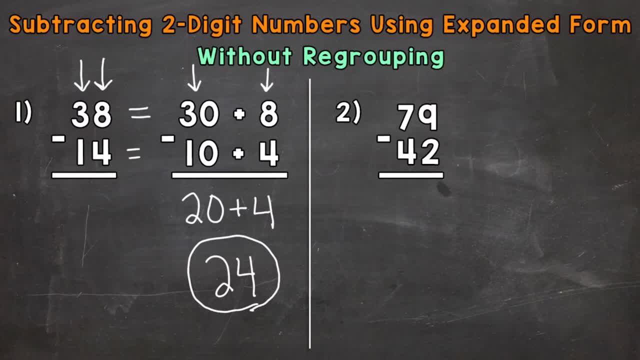 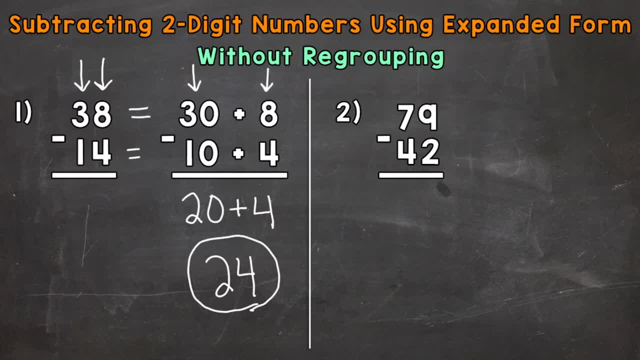 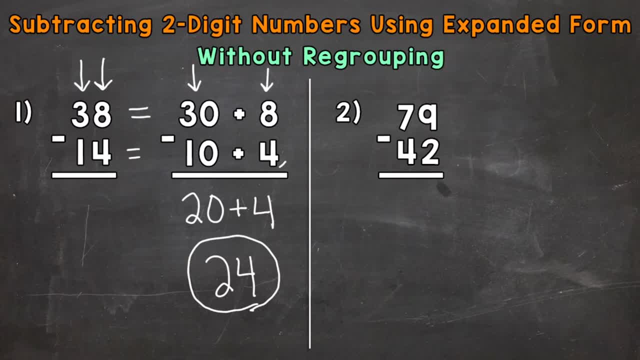 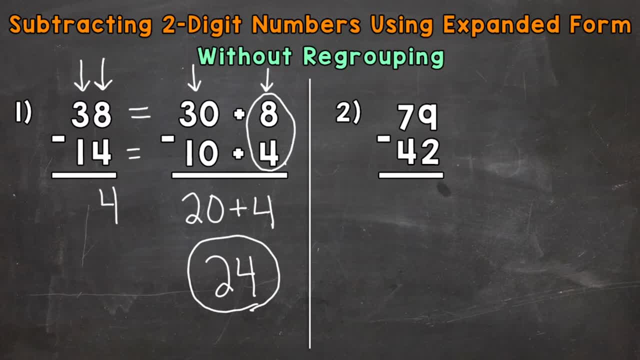 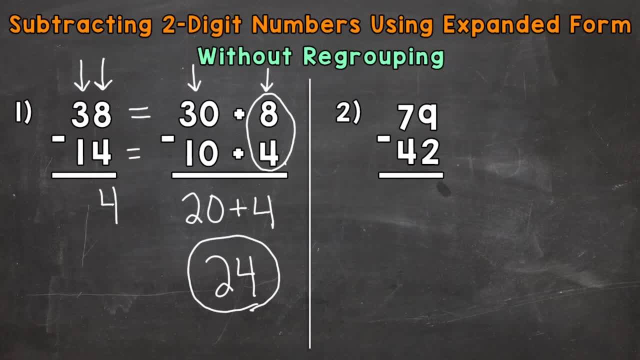 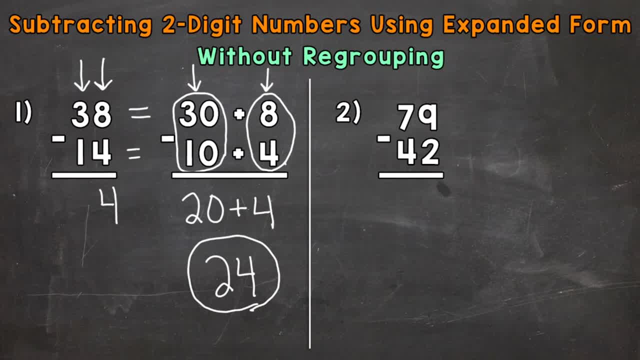 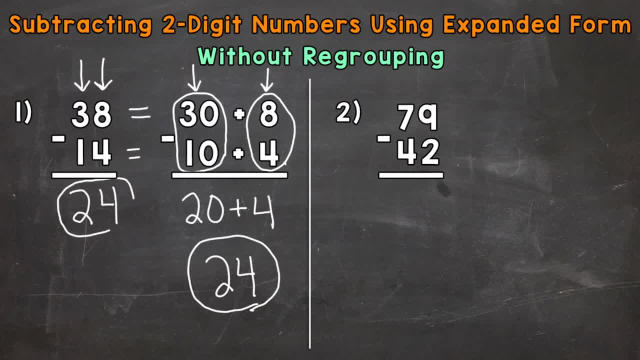 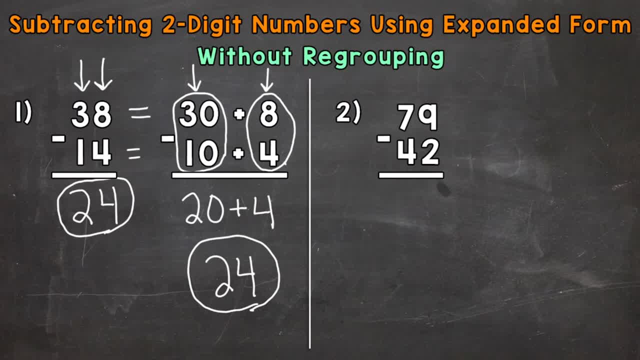 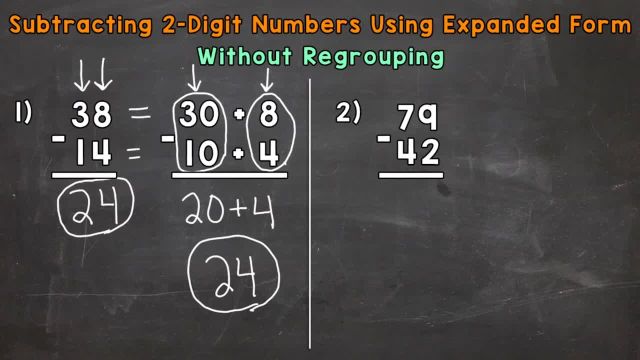 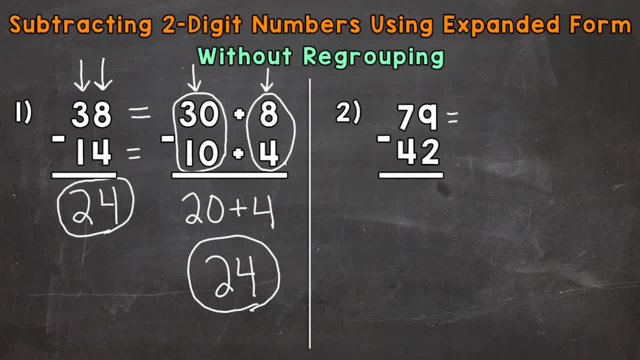 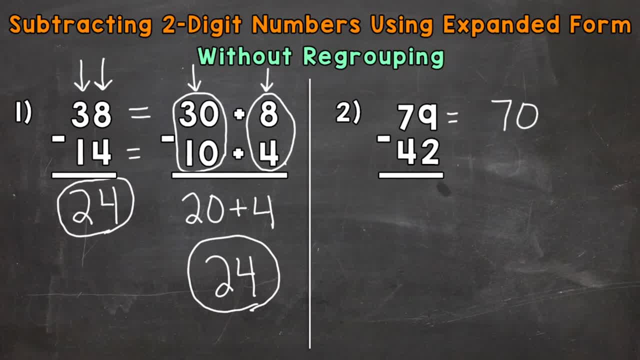 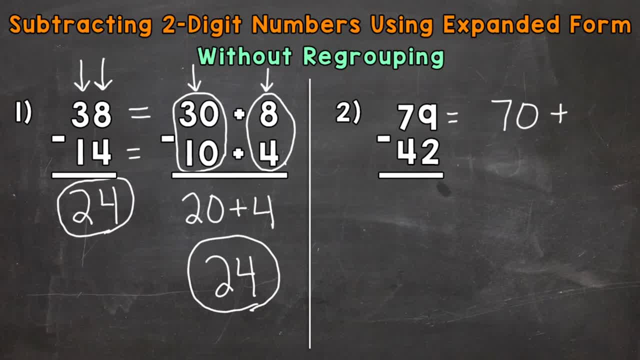 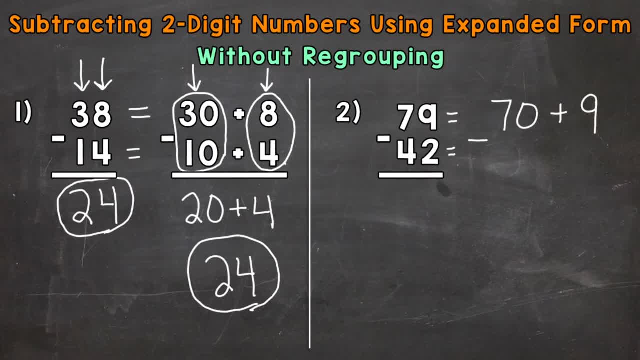 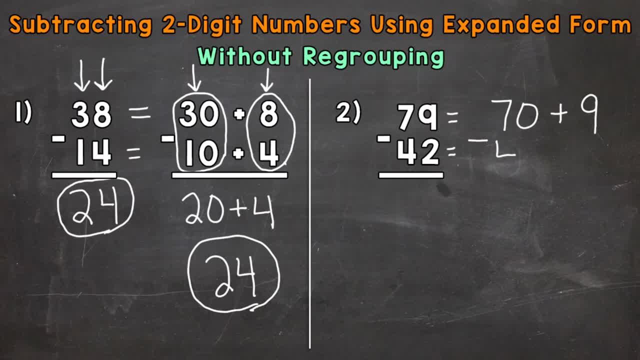 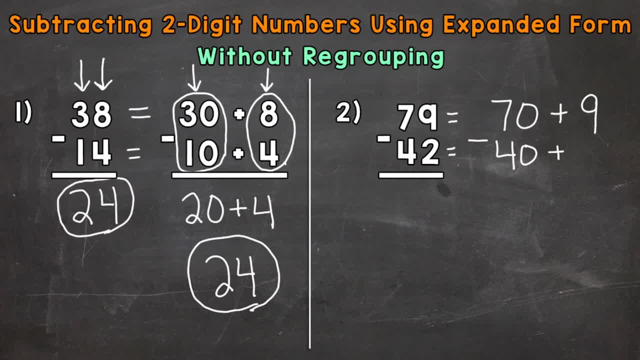 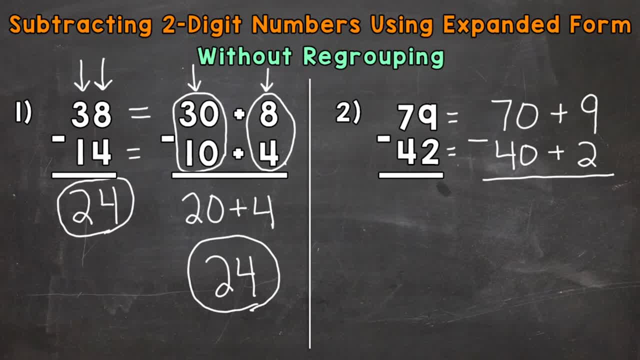 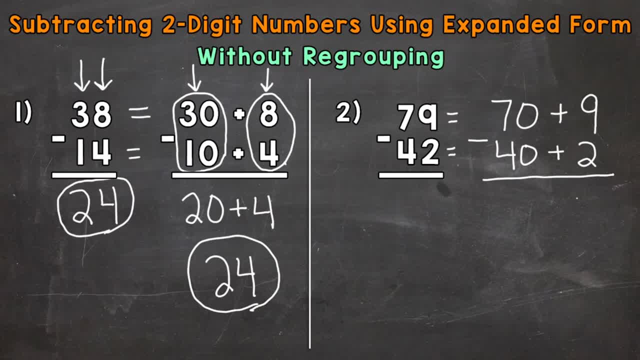 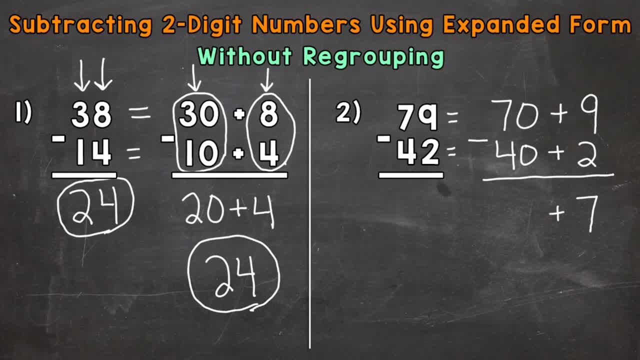 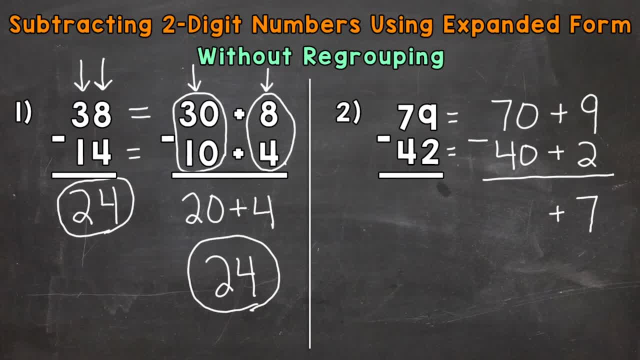 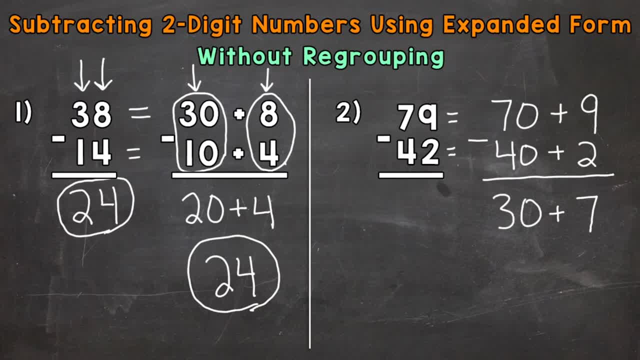 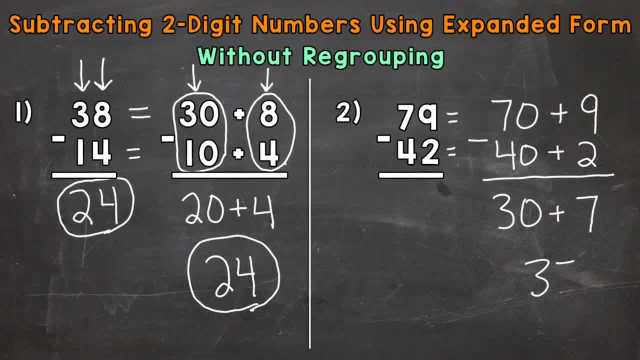 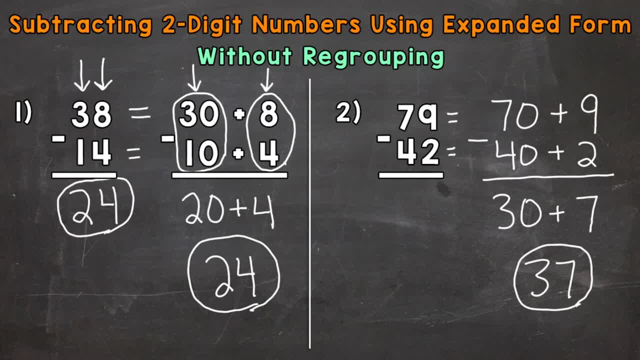 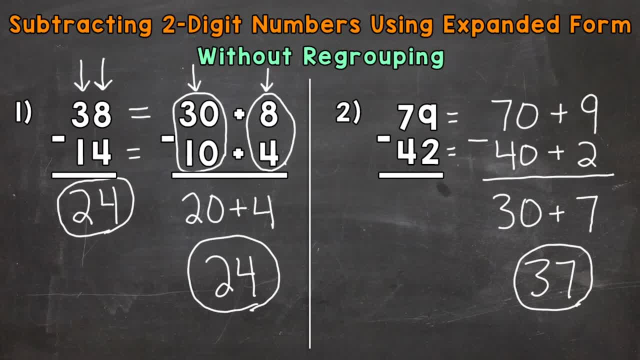 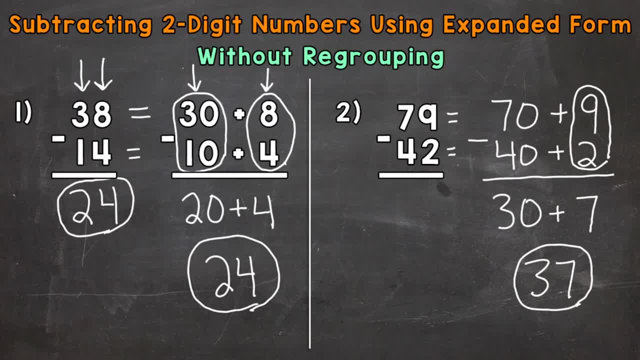 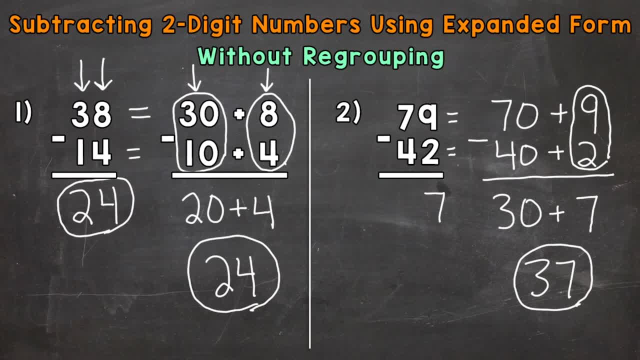 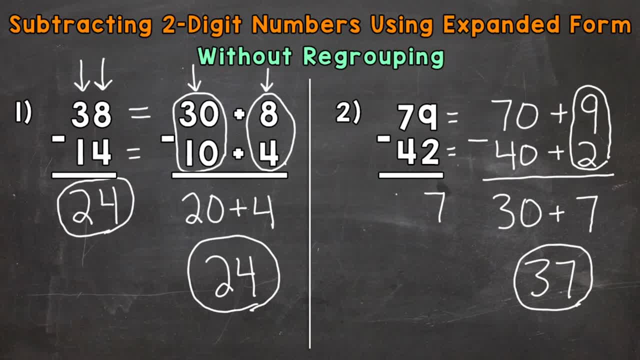 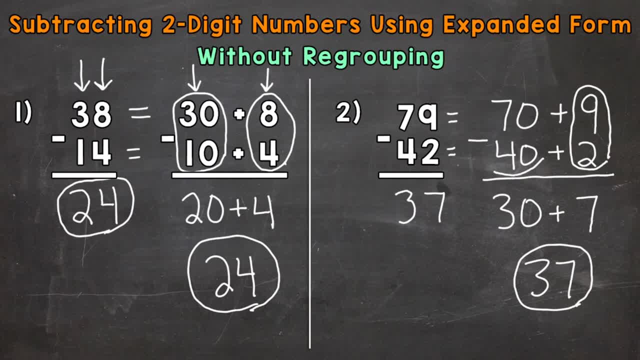 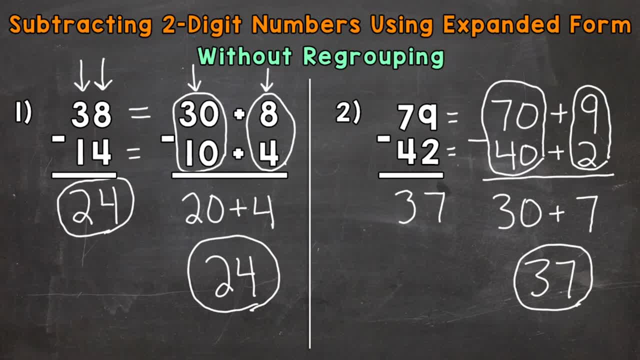 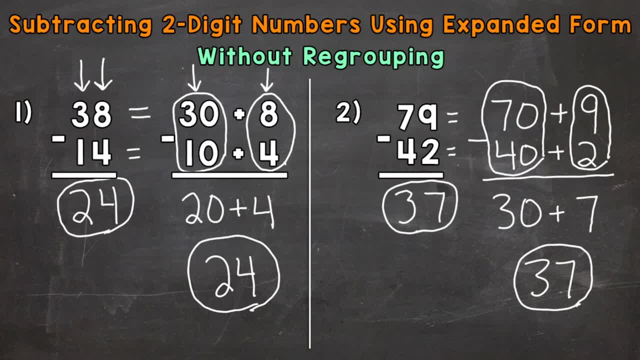 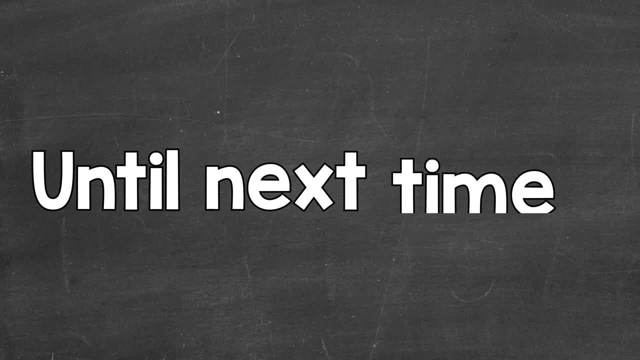 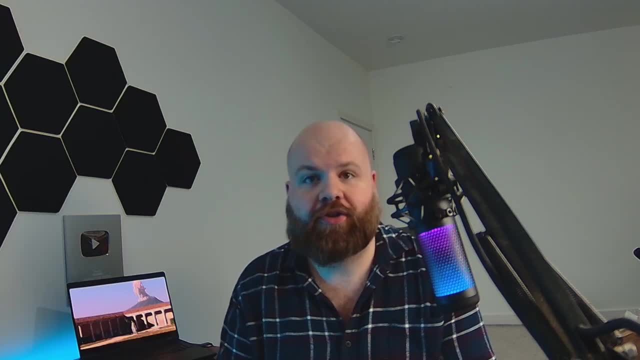 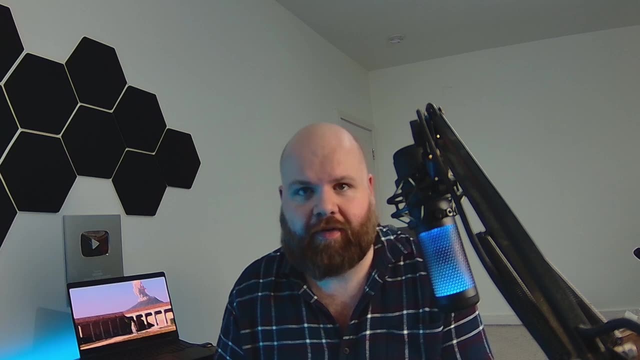 Since I made my last video about topology tips in Blender, I've had a bunch of requests to make some sort of follow-up, and I did promise a few months back that this would be a series. So luckily, I have quite a lot of these tips up my sleeve, so let's take 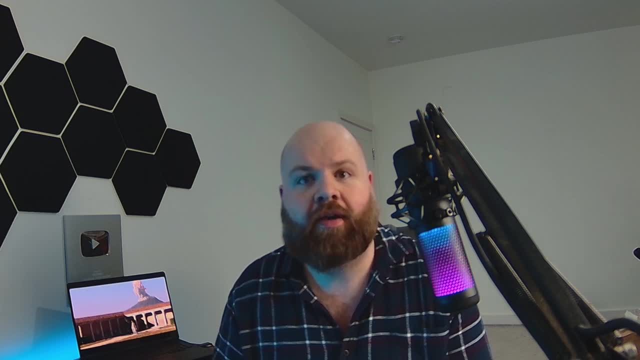 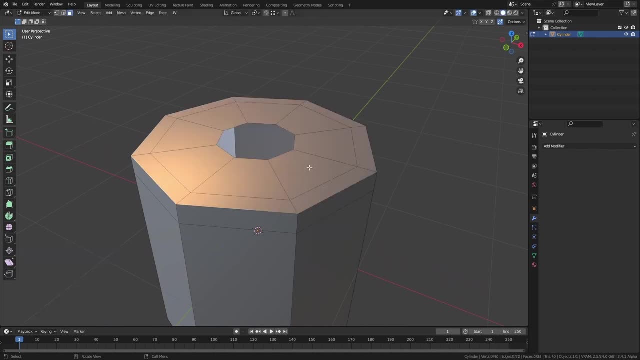 a look at some of the methods professionals use to handle their topology when 3D modelling. So at the end of my last topology video I showed off a method to create a cylinder that has all quads and no n-gons on the cap. A lot of people said they found that really. 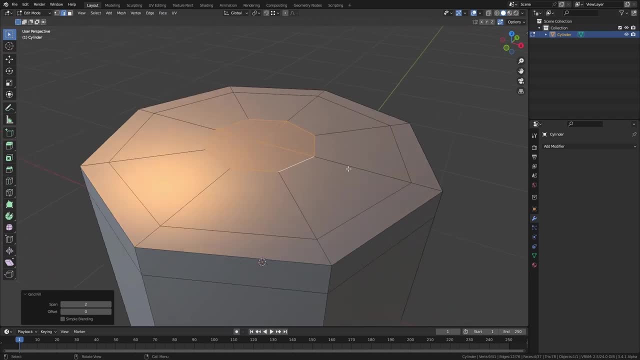 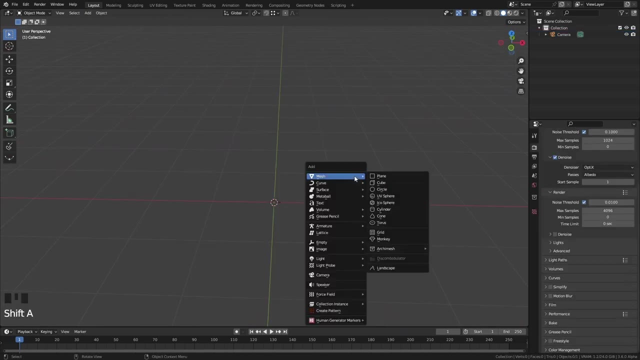 useful, and there's actually a few methods of doing this, with various strengths and weaknesses, so I thought I would show off a few of the methods that I commonly use. So the first method is essentially the same as the one I demoed in the last video. You